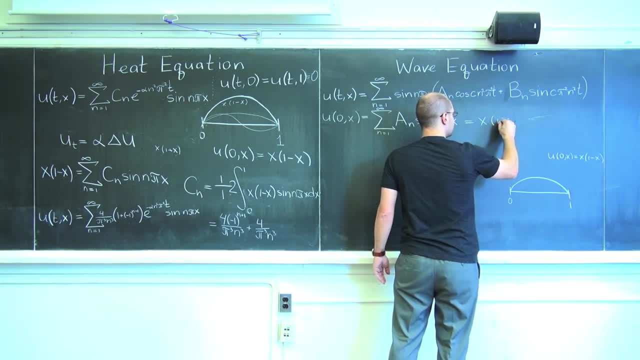 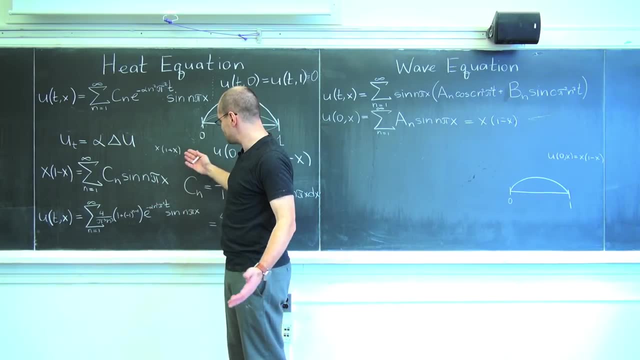 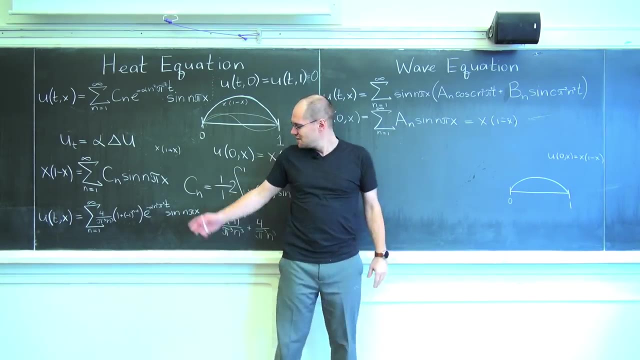 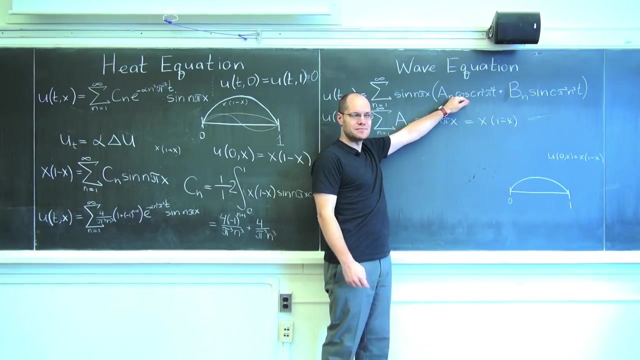 condition Equals x times one minus x. It should match the initial condition, And just like here, actually, I believe the problem is identical. It is, of course. We will get the same coefficients for a sub n's that we got here for c sub n's. Here we go, So that will give us a sub n's. 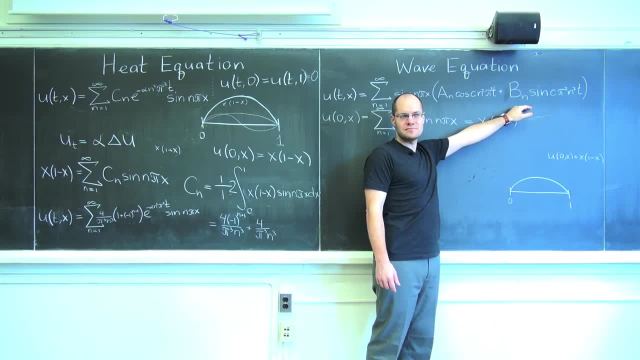 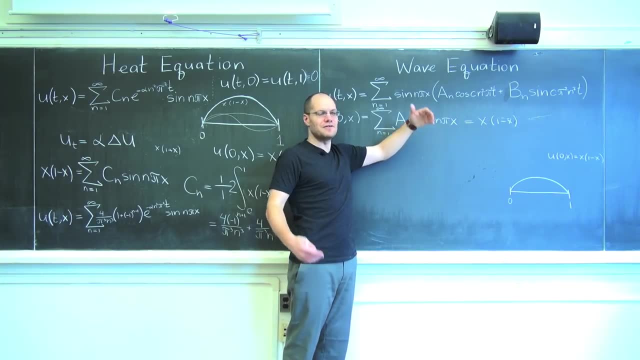 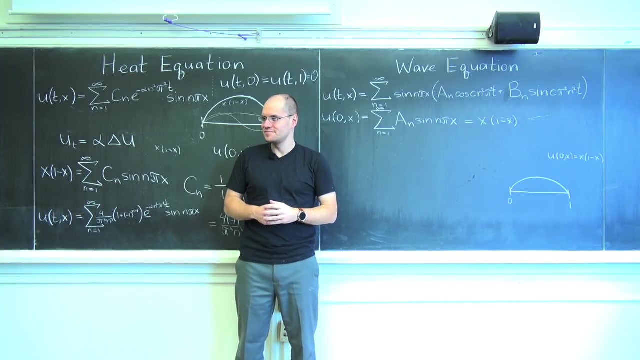 But what about b sub n's? Well, this is where you remember that this is an equation that describes dynamic evolution. It's Newton's law And with Newton's law, the Newtonian paradigm is that you indicate the initial location, but also the initial velocity. So when I said you pull on the guitar string and let it go. 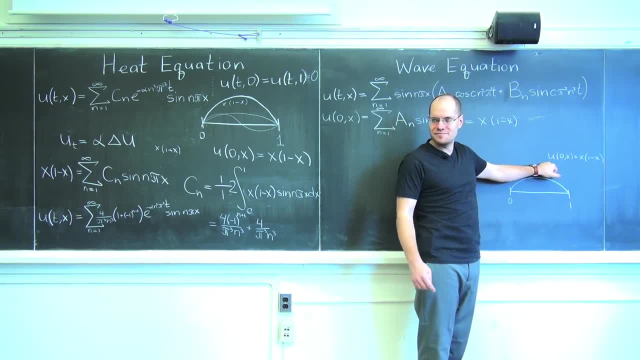 well, maybe that's the case where the initial velocity is zero, But if you strum, then at the moment you let go, the string is moving already if you strum quickly. So there is an initial velocity. of course We're missing one initial. 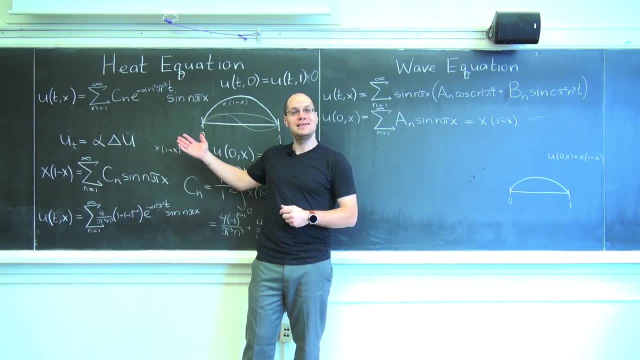 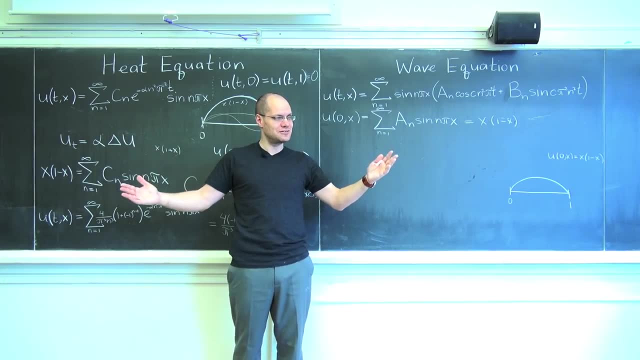 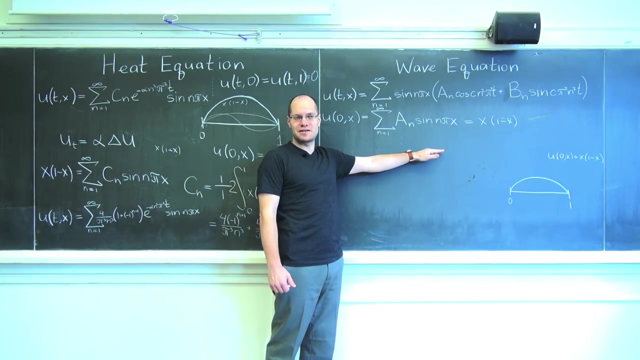 condition, Whereas the heat equation- you only need one, because you start with some heat distribution and then it relaxes to equilibrium. There is no inertia, There is no momentum. This is a much more lively equation. It's a dynamic equation. Some people use the term 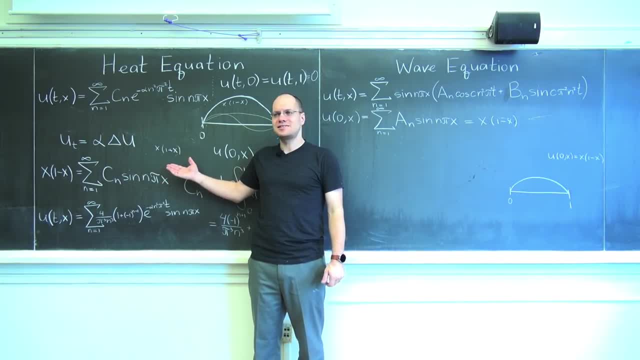 quasi-static, And quasi-static means at every moment it's really not moving anywhere, kind of Moving slowly Somewhere, But it goes whatever. Quasi-static, No inertia, But here it's all about inertia. And when there's inertia there is acceleration. And when there's acceleration there's second order. 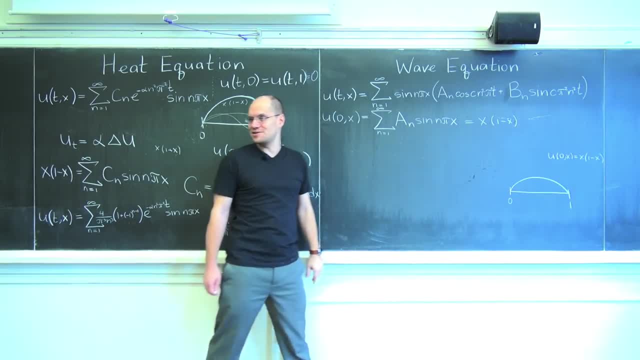 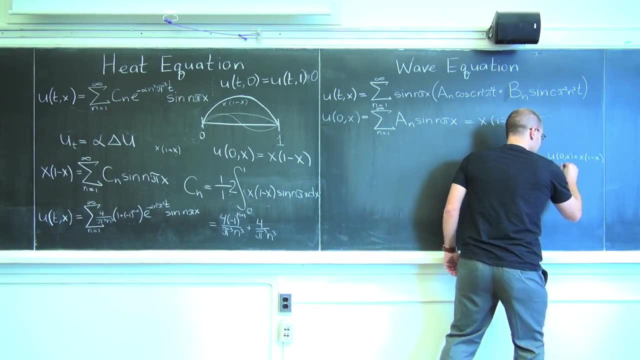 derivatives in time And when there's that, you need two boundary conditions, So of course you also need a velocity. What is velocity? Velocity is just the derivative with respect to time of u. So that's the sort of conditions that we're going to want to. 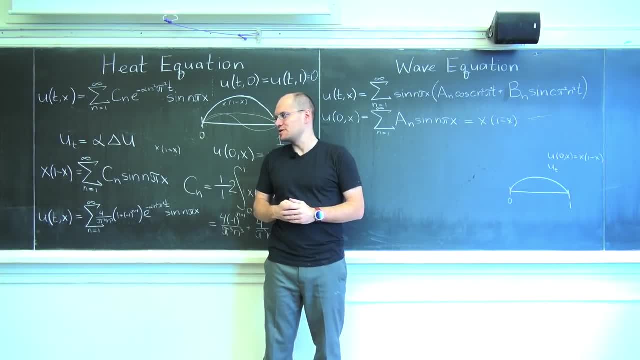 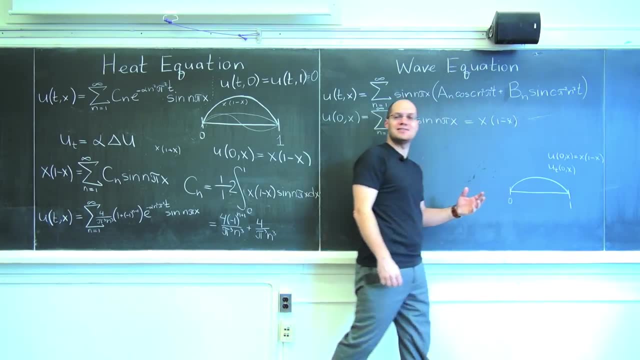 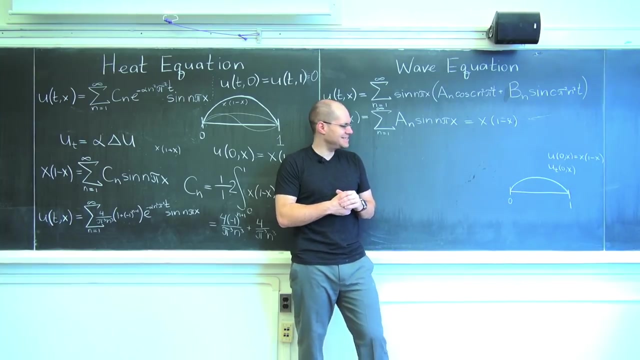 of conditions that the wave equation comes with, And you need to specify it at the initial moment, So you not only have to say where the string is, but how fast it's moving. Okay, what function should we choose? I don't know. 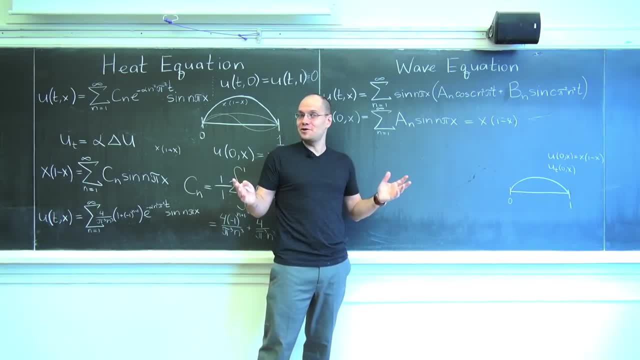 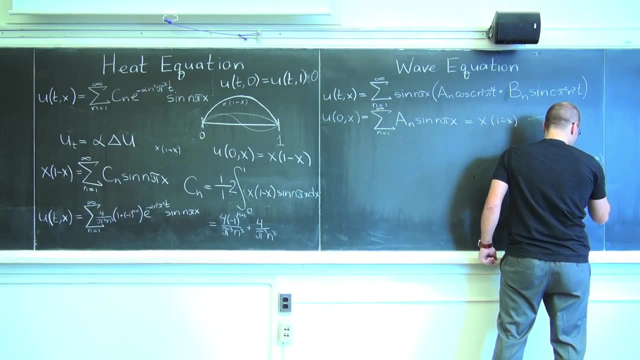 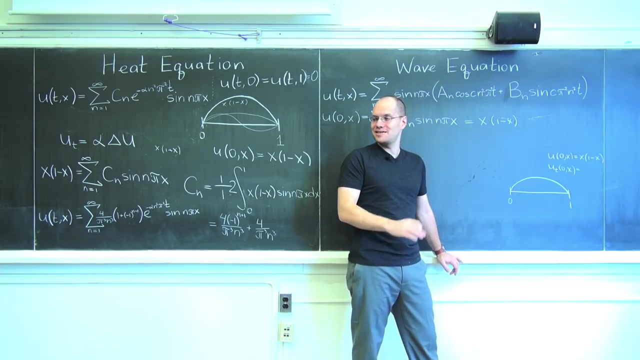 Let's choose. do we feel like evaluating more integrals? Yeah, I think we kind of do, So it will be. how about I just square this? eh, Why not Just to make it different? Or should I just? I could just make it x squared. 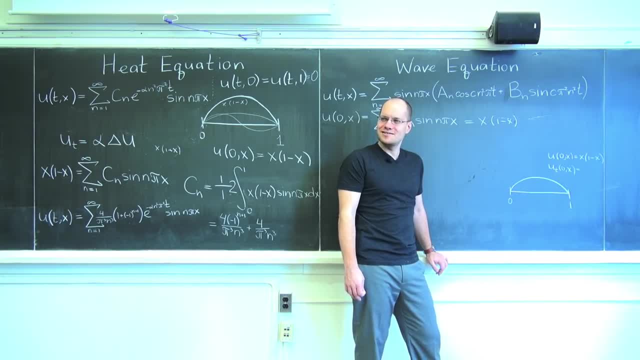 What would that do? That's a weird initial velocity, isn't it? But I just want to have something different. I could make it minus sine of pi x, but that would be a boring. Fourier series: All right, we're going to use Wolfram Alpha again. 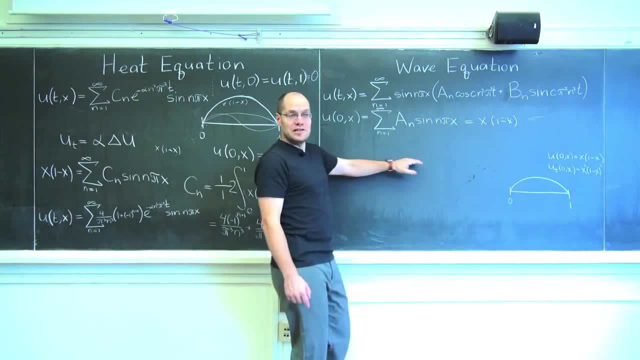 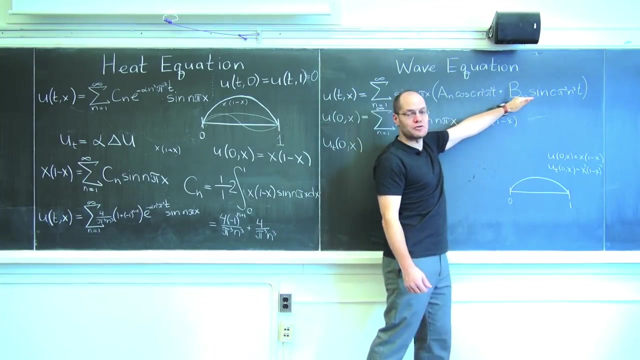 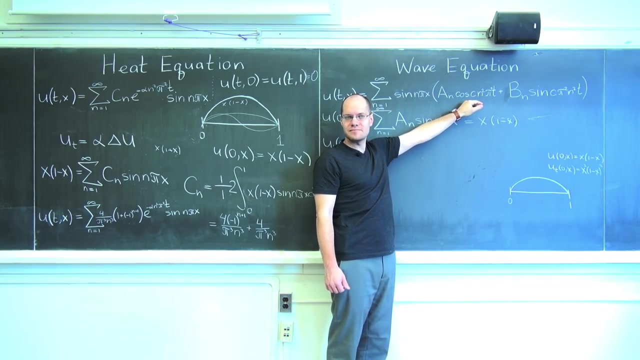 We will just fail. maybe a little bit later, Okay, but we need to do a little bit of work, because we need to see what the derivative will be, and so the derivative with respect to time only come from these terms. that's the only place where time appears, and this cosine will become sine, so 0, so 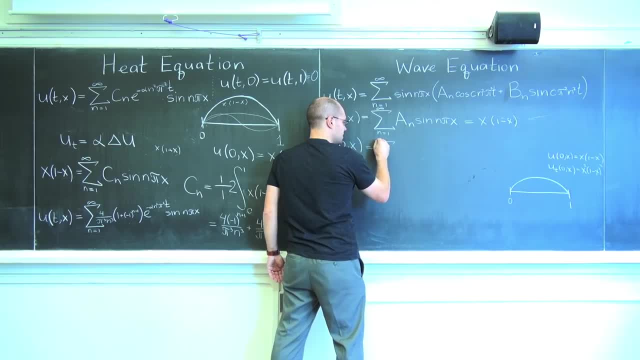 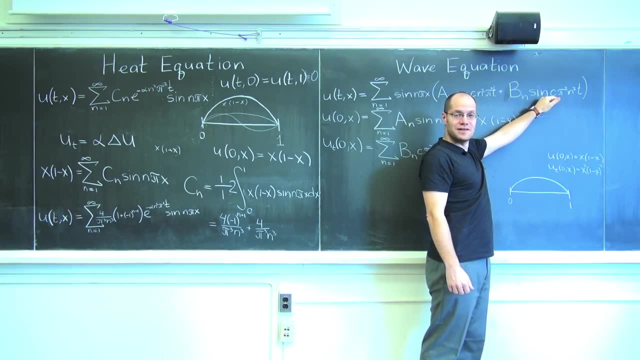 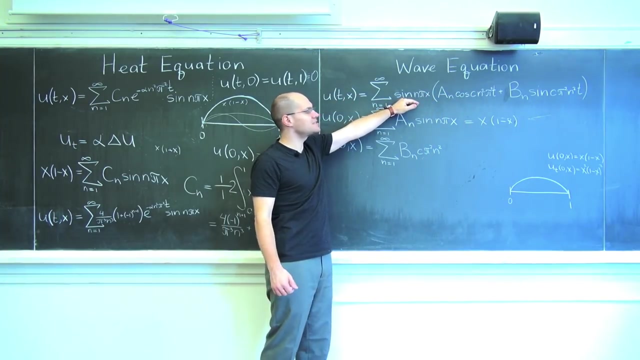 we'll just be left with b sub n's, so it'll be the sum and then cosine of this which we, when we plug in 0, will be 1. so that's good. so there's nothing left to do there. that's just 1 times sine and pi x. 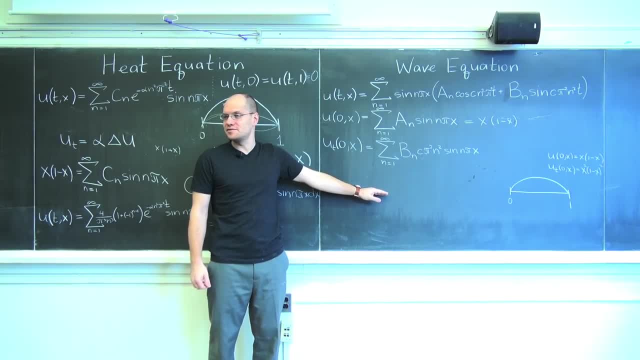 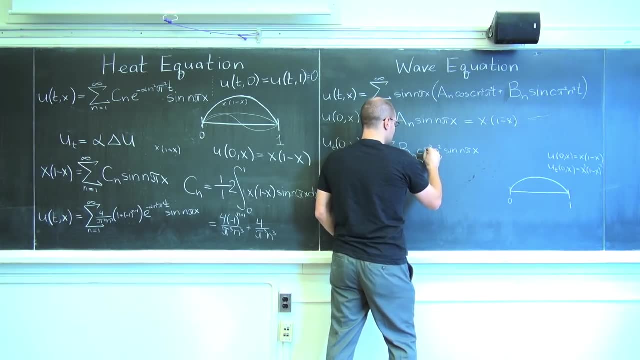 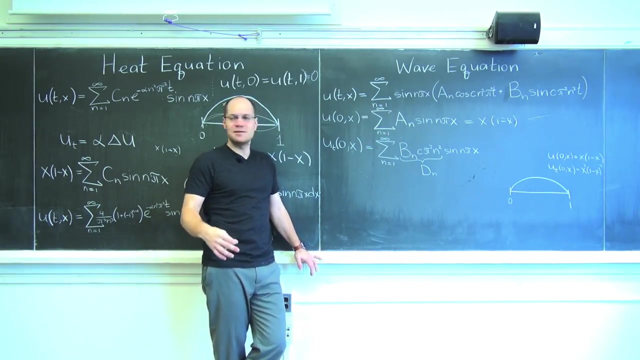 and there we go- pretty much the same series, except I will now give this combination a name to make Alex's life a little bit easier. we will call this d sub n. Alex will tell me what d sub n is and we'll get b sub n from it by. 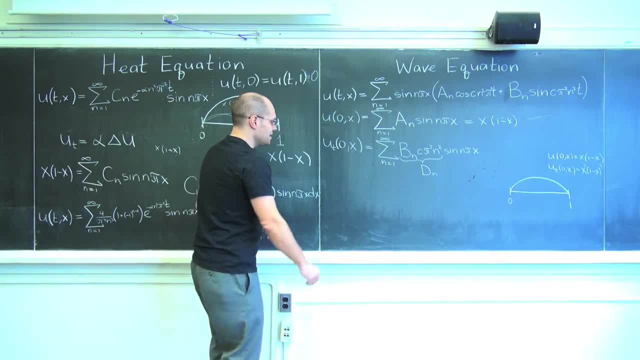 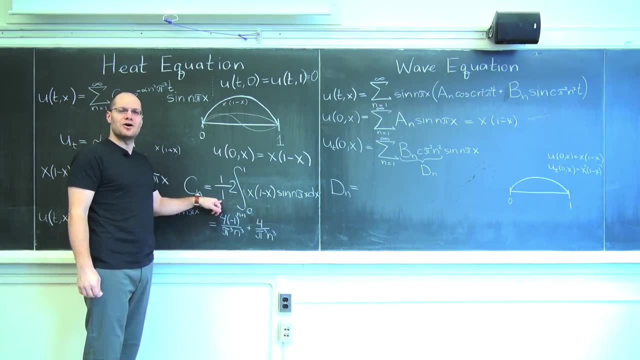 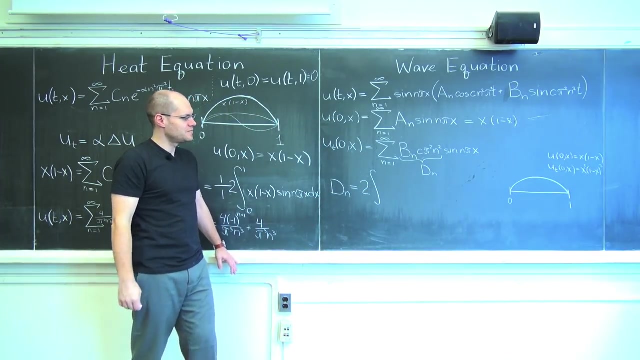 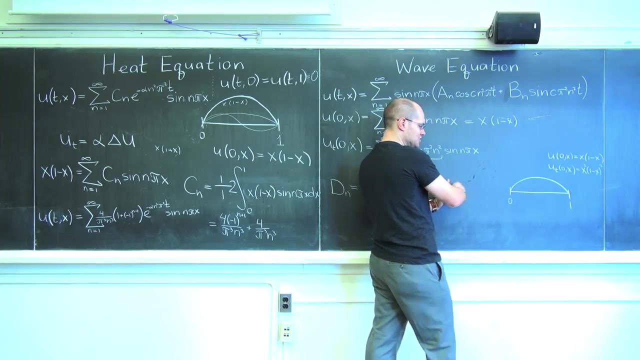 dividing by this. okay, let's write down what d sub n is. it will be this coefficient of 1. what is it? 1 over length over 2 twice, because of the same argument as before. we're going to find the symmetric, the, I guess, anti symmetric- odd repetition of this.